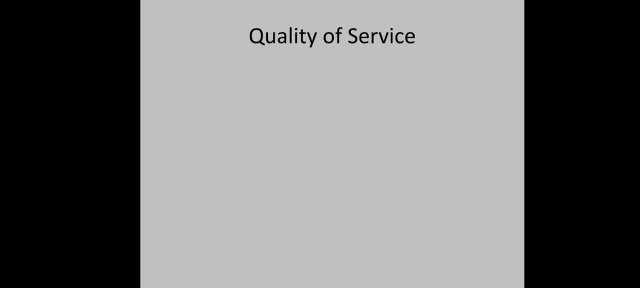 Welcome to the session on quality of service. In the previous session we went through some techniques to reduce the congestion and thereby improve the network performance side. However, with the growth of multimedia networking, the basic measures of service quality is not enough. but the applications are demanding for a good quality of service in any circumstance. 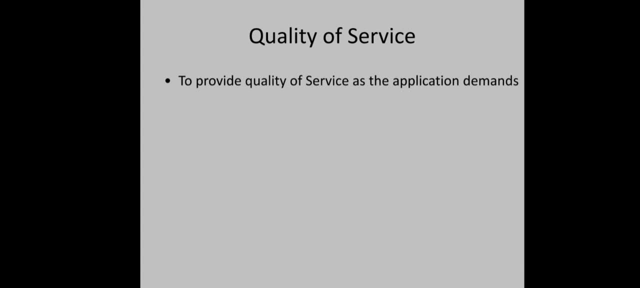 So now we will focus on how to provide a quality of service as per the application requirements. So before moving into that area, let us think: what are the different parameters which decide this quality of service of a network? So the parameters are reliability, delay, jitter and 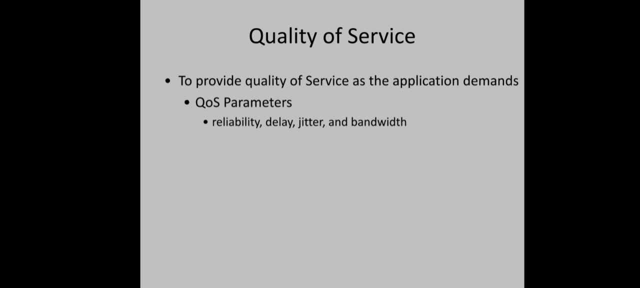 bandwidth. So these four parameters determines the quality of service offered by a network. So you are already familiar with reliability, delay and bandwidth. right, Jitter. we will discuss now And after that we will see different applications and what are the different. 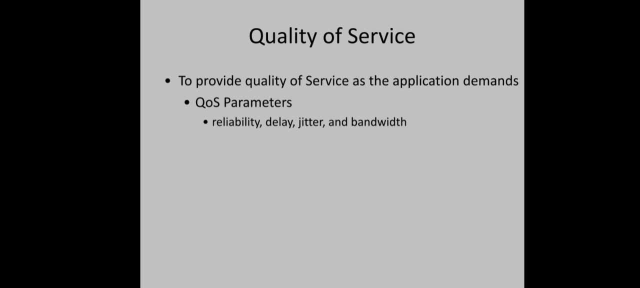 requirements faced by these different applications, on these four different parameters And finally, we will discuss different techniques to ensure that such a quality of service is provided, provided by this network to that applications. Now, the reliability determines how much error free the network is, Delay determines how fast is the network and the bandwidth determines how. 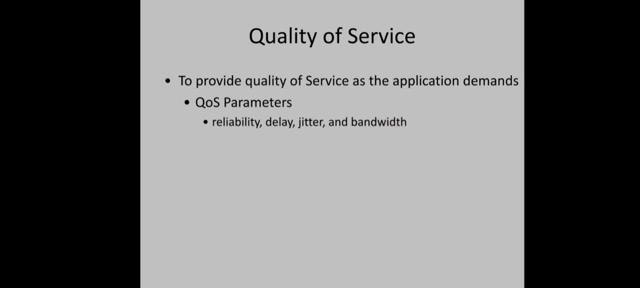 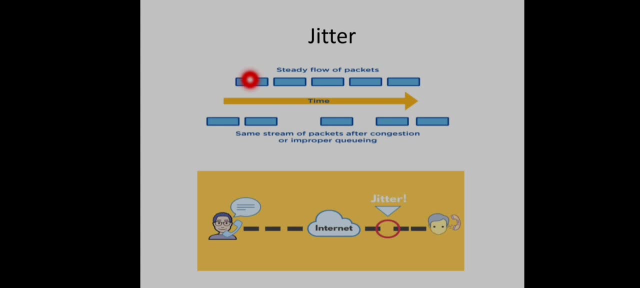 many bits can be sent per second over the links And coming to jitter. jitter is the variation in the packet arrival time, Just for example. here you can see there is a steady flow of packets. Between every pair of packets the gap time gap is the same right. Usually the sender will send. 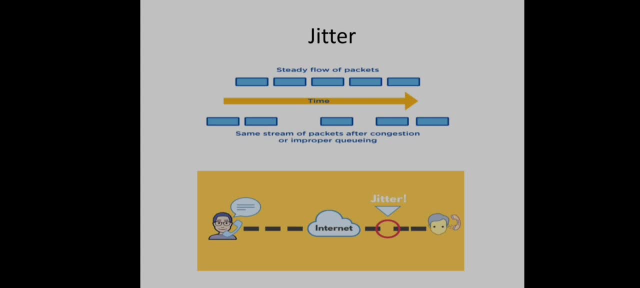 the packets to the sender And, due to some congestion, and all at the receiver. the data packets may arrive at different times And the time gap between these successive packets may be different. The variation may be different. Just for example, here you can see that the first and second 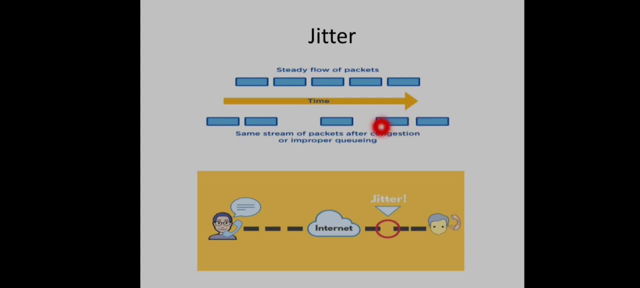 packet there is only a small gap, maybe one millisecond, And between this second and third packet the time gap is more right, Maybe four milliseconds, And here from third and fourth it is about, say, 10 milliseconds. So this variation is actually quite significant. 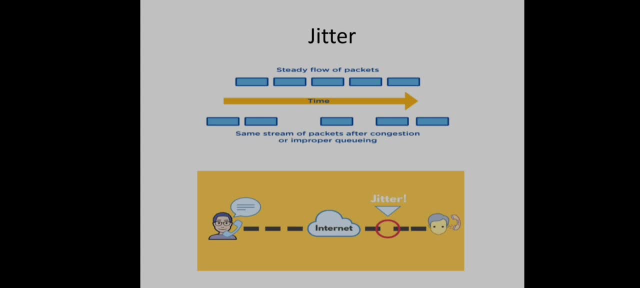 And the effect of this jitter is different in different applications, right? Just for example, some real-time application. Suppose we are talking on the phone and there is high jitter and the first word reaches in time, the second word reaches after, say, one second, and the third 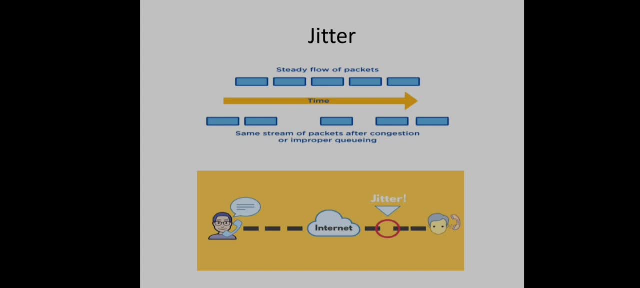 word reaches after three seconds, In that case the conversation will be annoying, right? So in that case jitter is having a great effect, Whereas in some other applications, like fire transfer and hold, this jitter is having not that much effect. 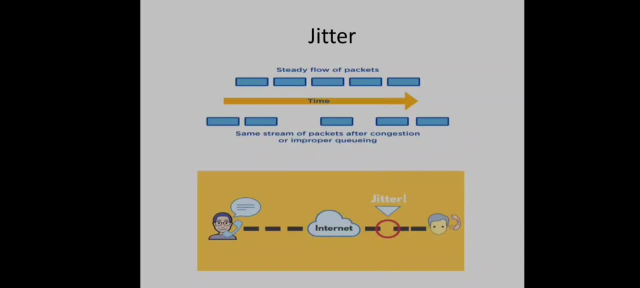 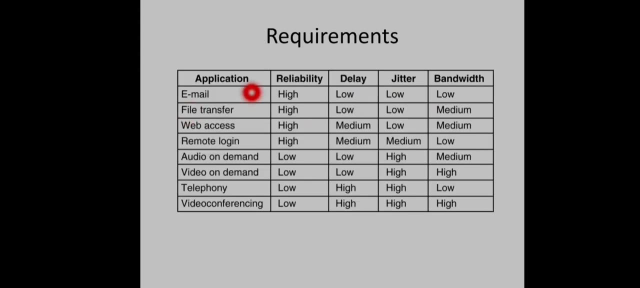 Okay, so we will see what are different applications and their corresponding quality of service requirements. Let us have a quick review of some of the applications, how these requirements differ. The first four applications: email, file transfer, web access and remote login. 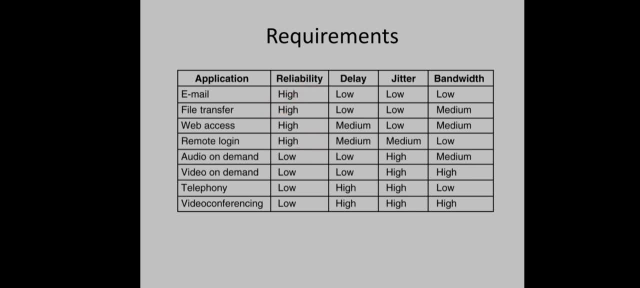 all these are having a strict requirement on reliability. So how to achieve this reliability? Of course, using the checksum and all we can achieve a good reliability right. So a checksum will be included with every packet and these will be verified at the destination. 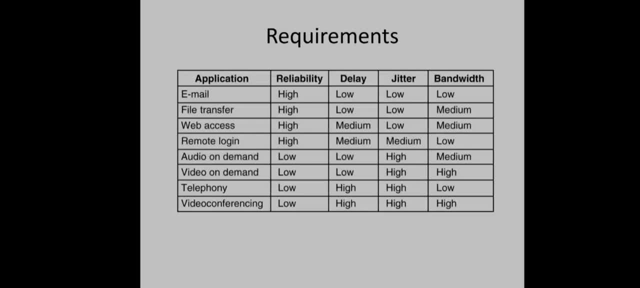 And if there is a mismatch, that corresponds to the quality of the service. And if there is a mismatch, that is because the corresponding packet will be retransmitted. By doing this, high reliability can be ensured, Whereas the next four applications- audio on demand, video. 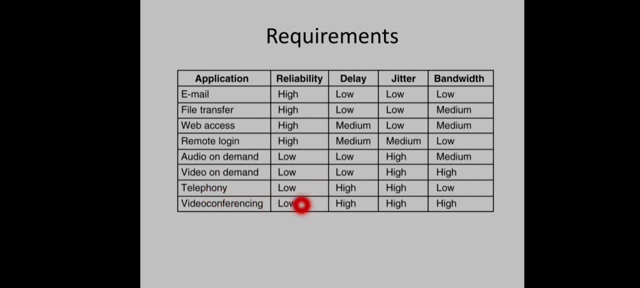 on demand, telephony and video conferencing. they can tolerate errors, right, So checksumming is not used here. Now the file transfer applications, including email, video on demand, audio on demand, etc. they are not sensitive to delay, right, If all the packets are delayed uniformly. 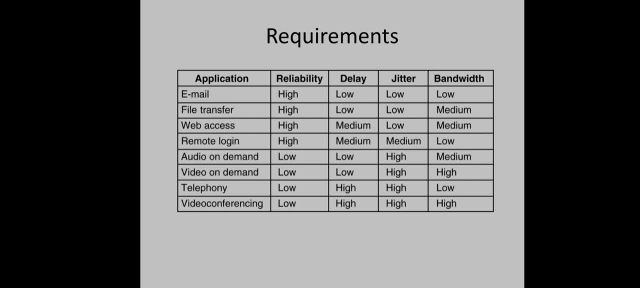 by a few seconds, no issues at all, Whereas the interactive applications like web surfing, remote login etc. bit more delay, sensitive, right, and what about jitter? yeah, the file transfer applications like email file transfer are not sensitive to jitter, whereas this remote login is somewhat sensitive. 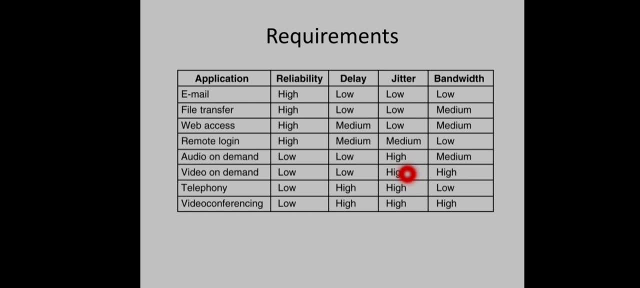 jitter sensitive right, whereas real-time applications like audio on demand, telephony, video conferencing and all are highly sensitive to this. jitter is, for example, if a user watching a video over the network and the frames are all delayed by exactly two second, no issues right. but if the transmission time varies randomly between one and two seconds, the result will be. 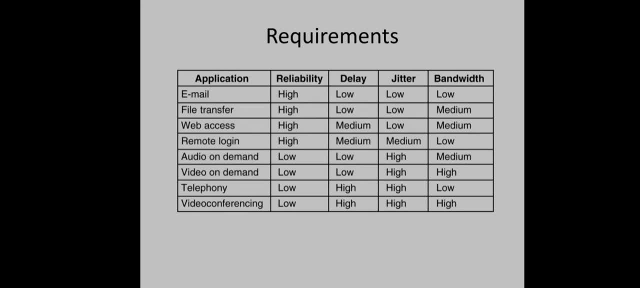 terrible for audio. the effect of jitter will be more. a jitter of even a few milliseconds will be clearly audible in case of audio. finally, the applications differ in their bandwidth needs. this, for example, with email and remote login not needing much bandwidth right, but video in all forms needing the bandwidth in a great deal. now let us see different techniques to achieve this. 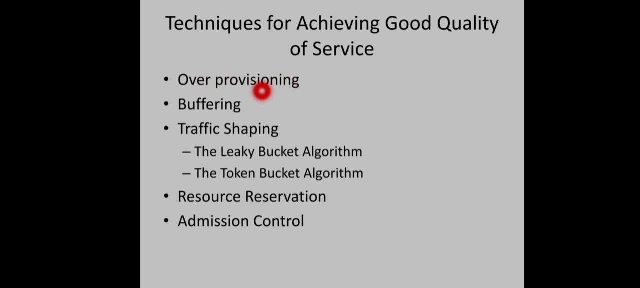 quality of service. so the techniques are over provisioning, buffering, traffic sharing and over provisioning the bandwidth in a great deal. now let us see different techniques to shaping resource reservation and admission control. so in this session we will see the over provisioning and buffering and the remaining we will see in the forthcoming sessions. the first: 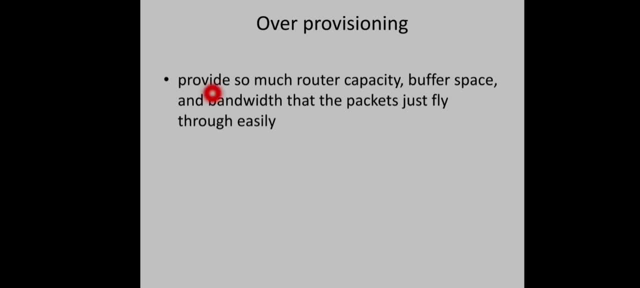 technique is our provisioning, as the name suggests, provides so much through tech capacity, buffer space and bandwidth so that the packets can just fly through this network easily. the problem with the solution is of course it's expensive. to some extent we can say that telephone system is actually. 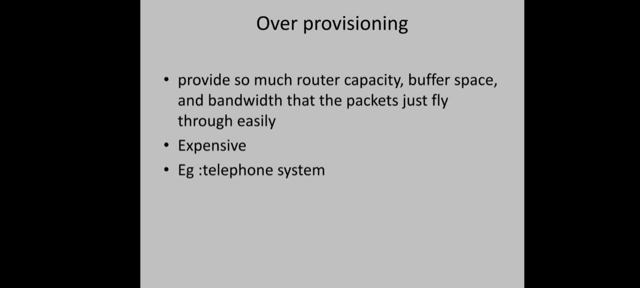 over provisioned. usually the chance of getting a network busy tone is rare in case of telephone right. if he calls, the telephone system is actually over provisioned. usually the chance of getting a network busy tone is rare in case of telephone right. if he calls someone, usually we will get the dial tone itself. this is because so much capacity is available there. 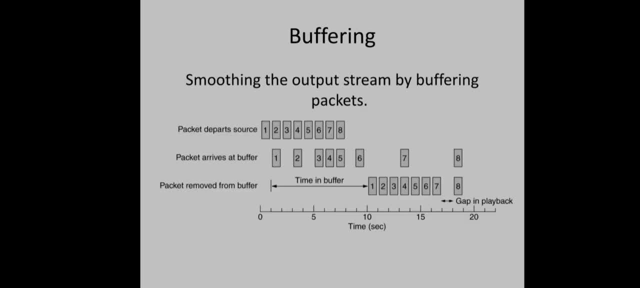 that the demand can always be met. and next solution is buffering. so in case of this buffering techniques, the data packets can be buffered on the receiving side before being delivered. so of course, this buffering will not help in reliability or bandwidth, right, it won't increase the reliability or it. 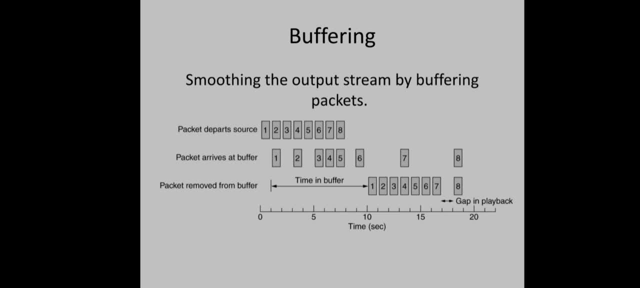 won't increase or decrease the bandwidth. surely it increase the delay, right, because the packets are getting buffered in the receiver before delivery. but it definitely smooths out the jitter. that's the benefit here. so jitter parameter is improved using this buffering technique for audio and video on demand. jitter is the main problem right there. this technique helps. 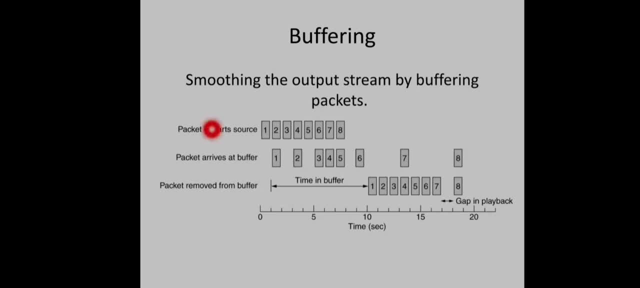 a lot. so we can see an example here. you can see here: there's a continuous flow of packets from the sender, but these packets are being delivered with substantial jitter. you can see here the time gaps. the time scale is in seconds. the packet one is sent from the server at time zero, zero second and 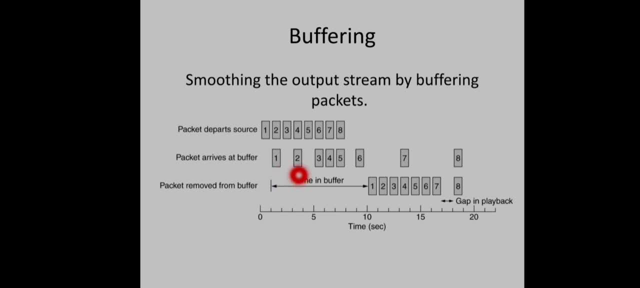 arrives at t equal to one second packet. two under goes more delay right and takes two seconds to arrive at the destination. as a packet arrive, they are buffered on the client machine instead of delivering every packet as it arrives. they are buffered in the client machine and the playback. 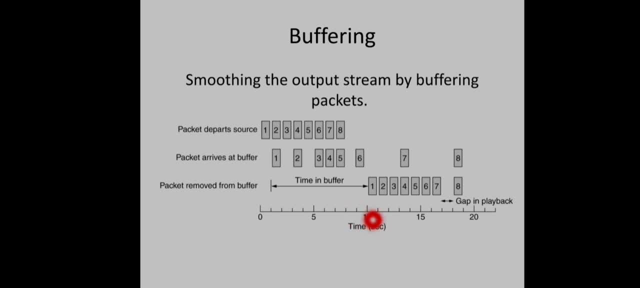 starts only at 10 second. okay, t is equal to 10 seconds. the playback begins at this time. packet one to six is already there in the buffer right so they can be removed from the buffer at uniform interval to smooth out. the communication at the time can be removed from the buffer at uniform interval to smooth out the. 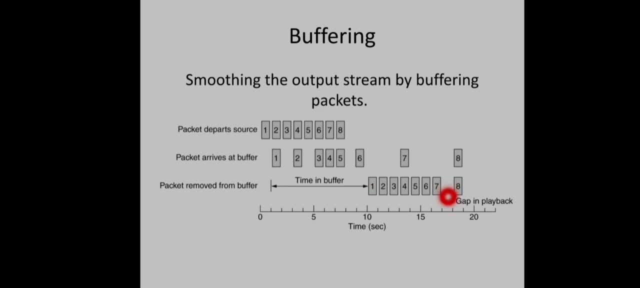 If we put packet 8, this uses slot for packet 8 in the playback, but packet 8 suffers a lot of jitter and arrives later only, So this will create an annoying time gap in the music or movie. This problem can be reduced by delaying the starting time even more, although this requires a larger buffer.